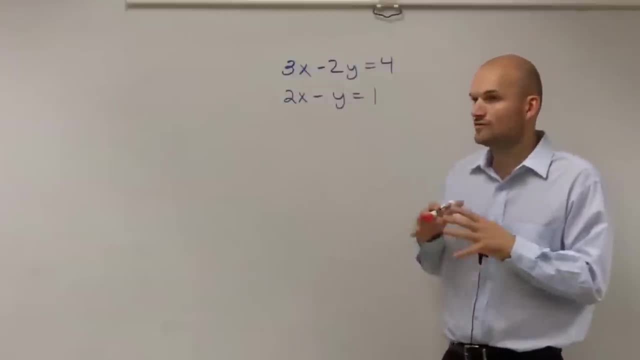 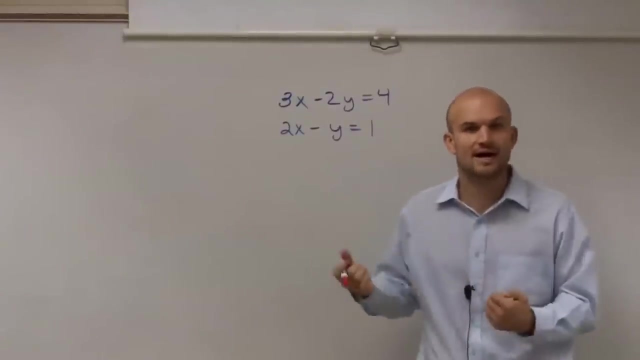 for solving systems. I am going to prefer to solve, set it into y equals mx plus b form, And the reason why is I can follow the slope to every single point that's on the line. so the intersection should be a little bit more clear for me, Because, remember, 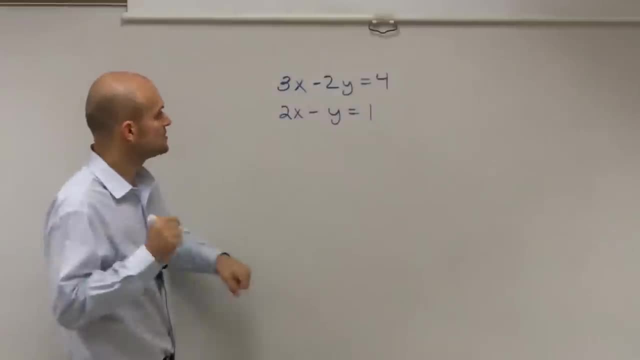 we want to find the x and y intercepts. We want to find the x and y intercepts. We want to find where these two lines intersect, if they do at all. So the first thing I'm going to do is I'm going to set up each equation and I'm going to solve. And I'm going to solve for y. 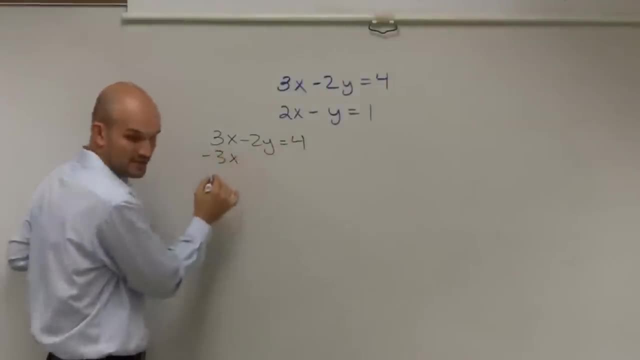 so it's going to be in mx plus b form. So to get y by itself I first need to subtract 3x on both sides, So I get negative 2y equals a negative 3x plus 4, right, We like to write the negative 3x. 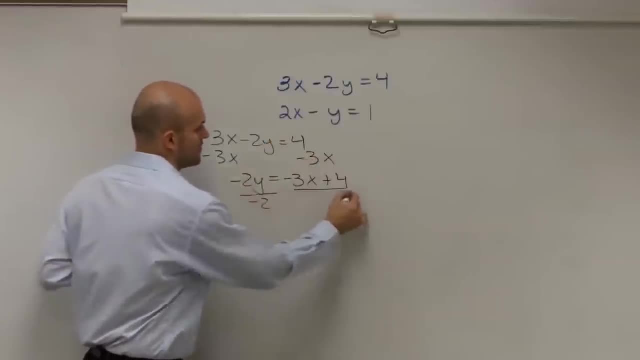 instead of the 4.. Then I need to divide by the negative 2.. So I have: y equals negative, 3x negative. 3 divided by 2 is a positive. 3 halves x. 4 divided by negative, 2 is a minus 2.. Now 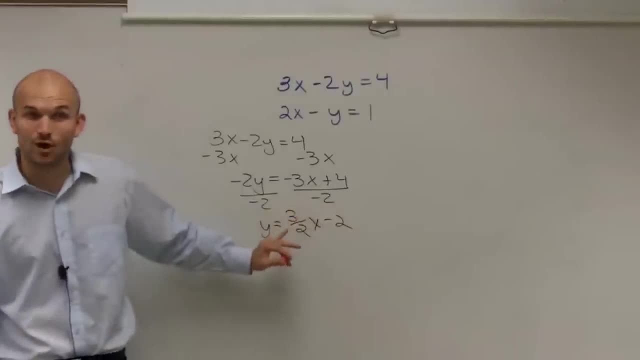 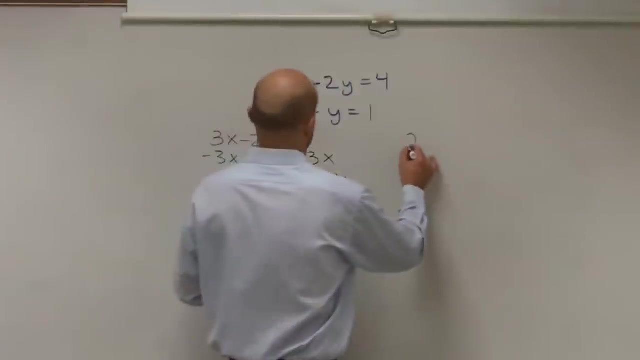 a lot of you might say, ooh, fraction, I don't like it. But remember, this is our slope, so this is actually going to be very helpful when we go ahead and try to graph this line. So the next one, let's write: we have 2x minus y equals 1.. Now I'm just going to get the y by. 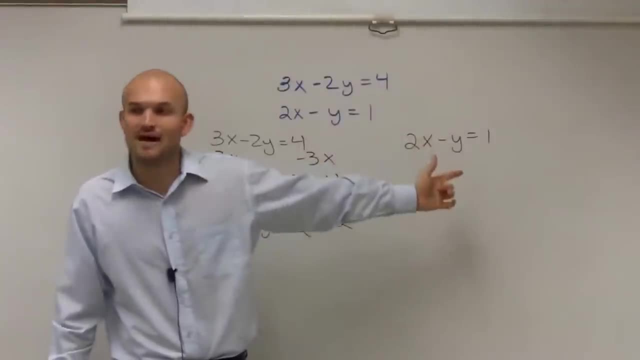 itself right, So I could subtract the 2x and then divide by negative 1.. However, for this problem, I'm actually going to add the y to the negative 1.. So I'm going to subtract the 2x and then divide. 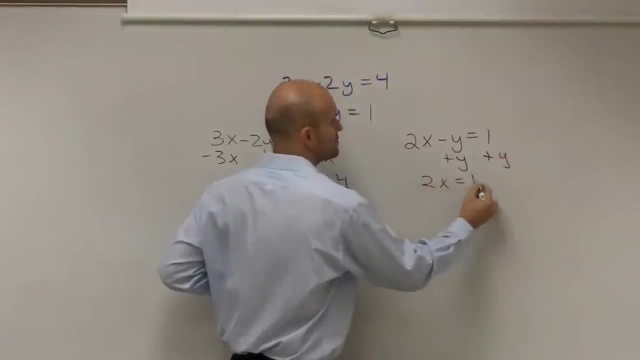 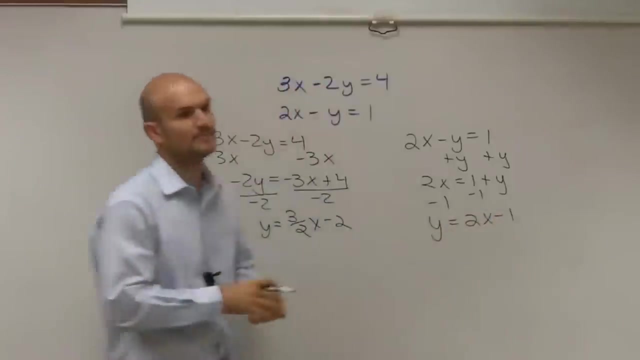 the y to the other side. So I have 2x equals 1 plus y, and then I'll just subtract the 1.. So my final answer is y equals 2x minus 1.. So now, how do you graph guys? how do you graph these two? 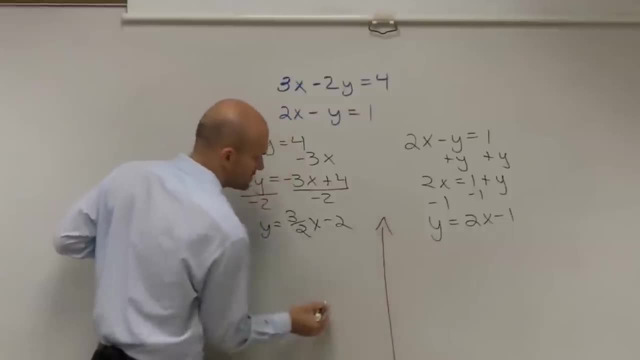 equations. Well, remember your equations. we're going to set up with an x and a y axis, all right, So remember when it's in y equals mx plus b form. we put it in this form so we can remember a couple things. This is your y intercept, right, And it's your y. 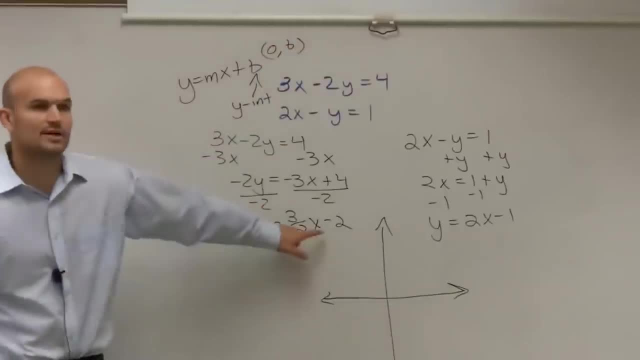 intercept at 0 comma b. So I'm going to go down. So I look at here and I say my y intercept's at negative 2.. That means this graph crosses at negative 2.. So I go down to negative 2,. 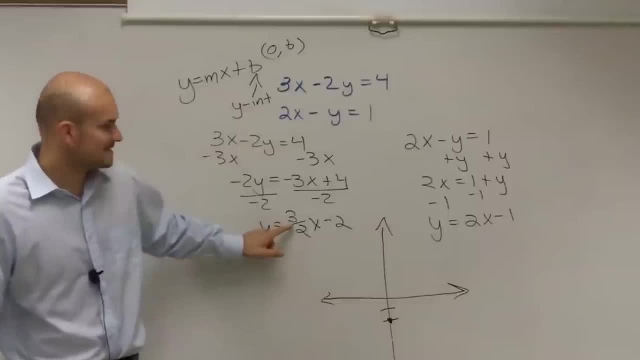 and I make a nice little dot. Then it says my slope is going to be 3 over 2.. And remember, because your m is your slope, Remember slope would represent like, as a rise over 1, it's the change in your y values. 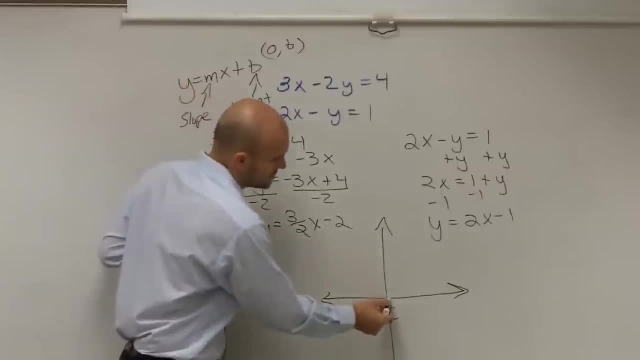 over the change in your x values. So I'm going to go up 3, 1, 2, 3, over 2.. So that's going to take me to my next point. You could also do a negative over negative. 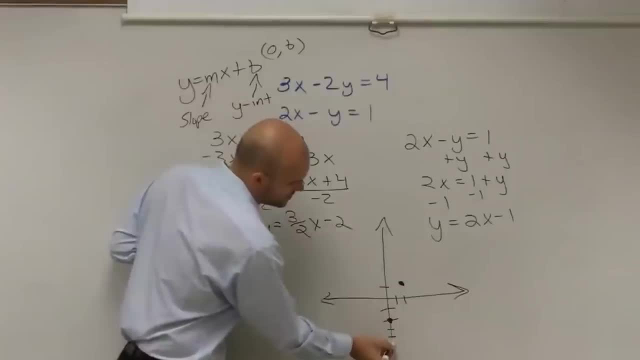 because that would still be positive. You could also go down 3,, 1,, 2,, 3, to the left, 2.. And then I connect my points and I have my line. Make sure, ladies and gentlemen, I've seen a lot of people graphing. 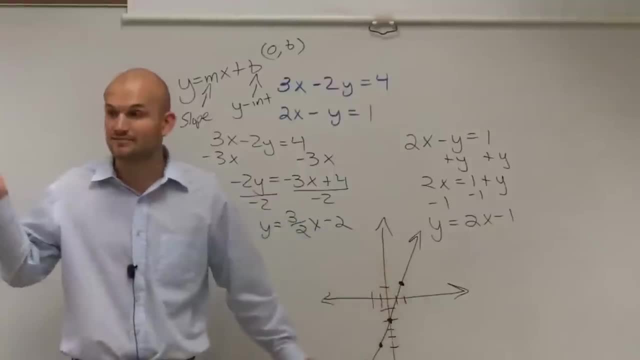 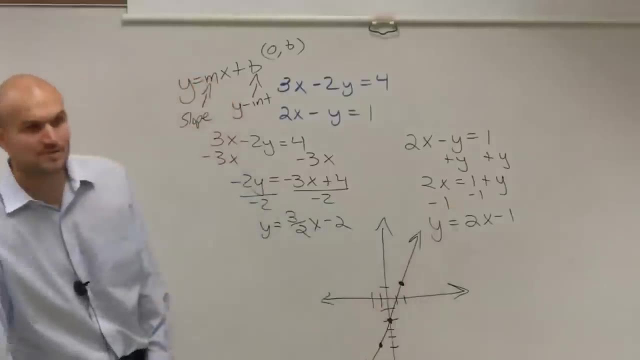 and they're not putting the arrows When we're graphing lines. they have infinite length, So make sure you create those arrows at the end. The next one: it says 2x minus 1.. So now this one goes down at negative 1.. 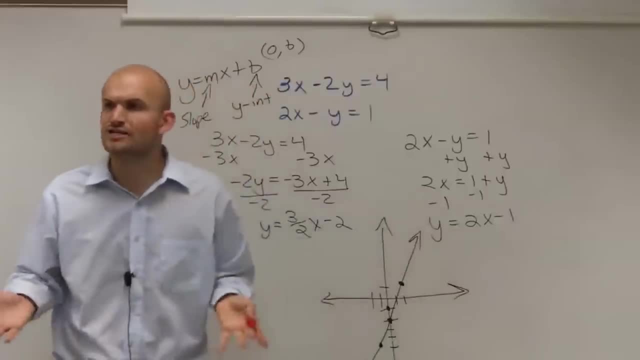 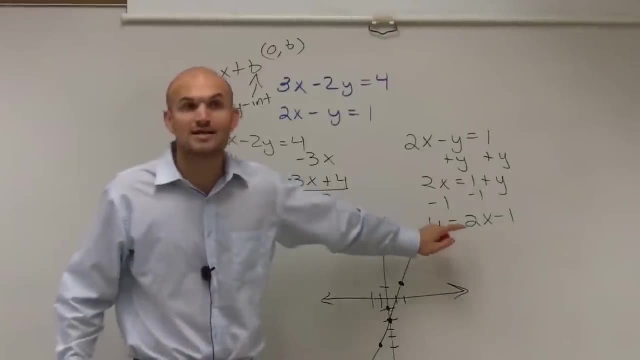 But my slope is a 2. Well, how do you do change in y over change of x? It's going to be your change. You need to make sure you have to write this as a fraction. So actually we're going to want to make sure. 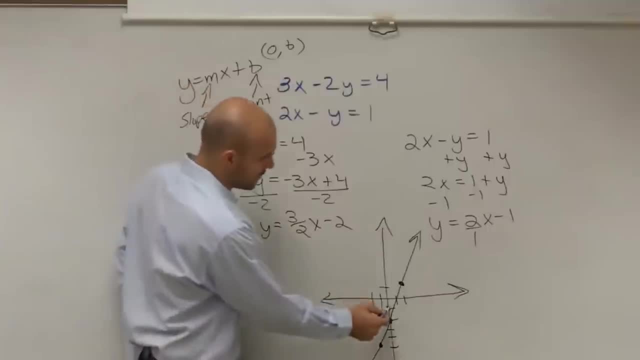 we write it as a fraction, with 2 over 1.. So, therefore, I'm going to go up 2 over 1. And if I keep going like that, I notice that these aren't going to graph. However, if I go down, 2 to the left, 1,. 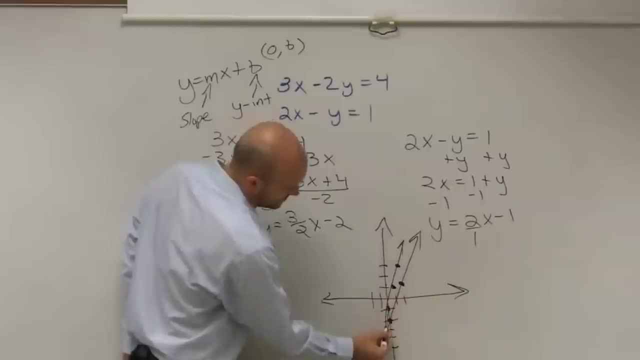 we notice that they- If my graphs are a little bit OK- Well, we notice that they intersect at a certain point. So what was that point? That point was at negative 1,, 2, 3 over 4.. So we could say the solution. 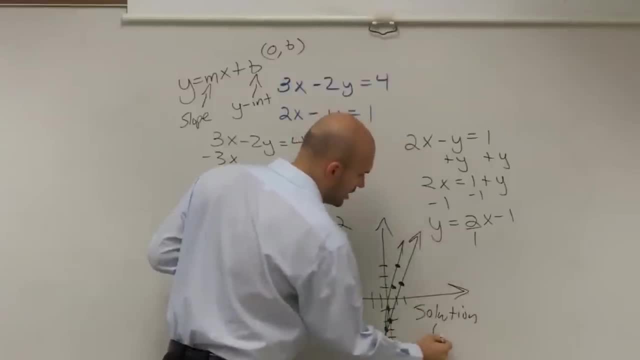 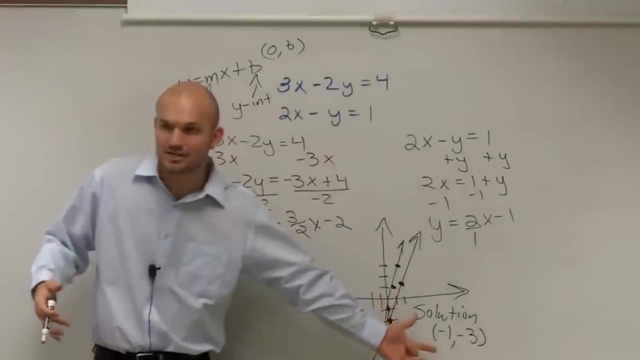 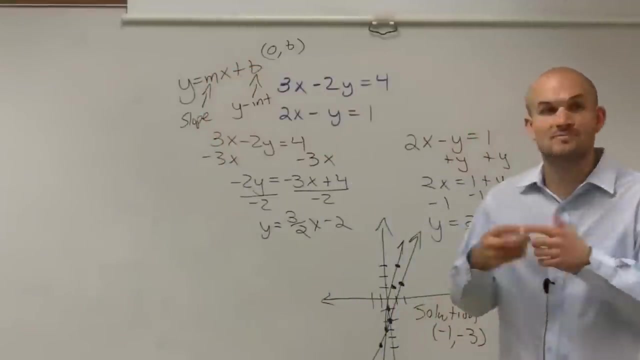 is at the, at the point of negative 1, comma, negative 3.. Because that is the intersection, All right. So then we look at our solution. Is it consistent or inconsistent? Since we have, Since we have a solution, it is consistent. 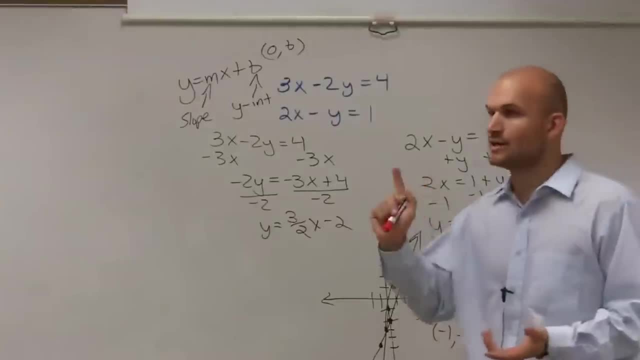 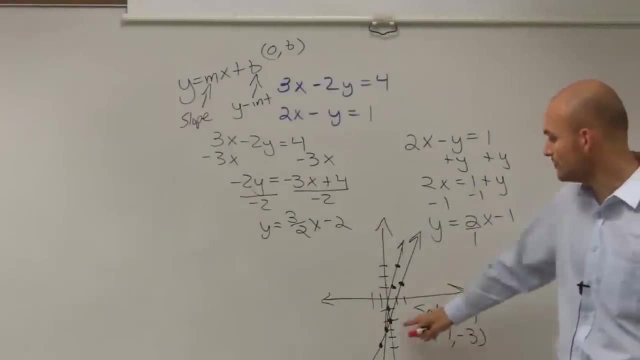 And then is it independent or dependent? Since we only have one solution, it is going to be an independent solution. So it's independent, consistent solution, And we can just write our solution as the coordinate point, Because at that coordinate point, 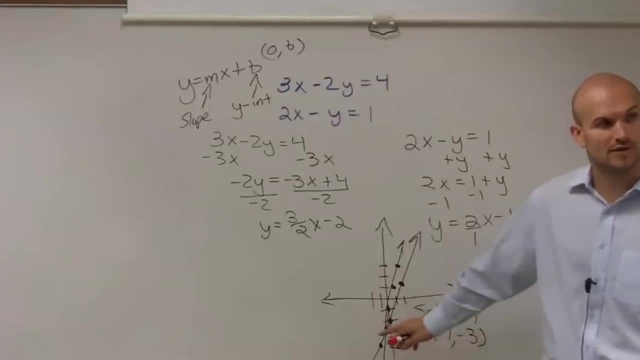 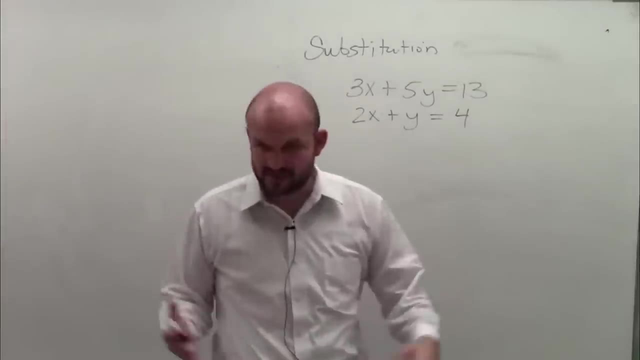 our two graphs are equal to each other For x and y. All right. So, ladies and gentlemen, what we have here is we are going to solve the system by substitution. Now, this we could solve by graphing right. 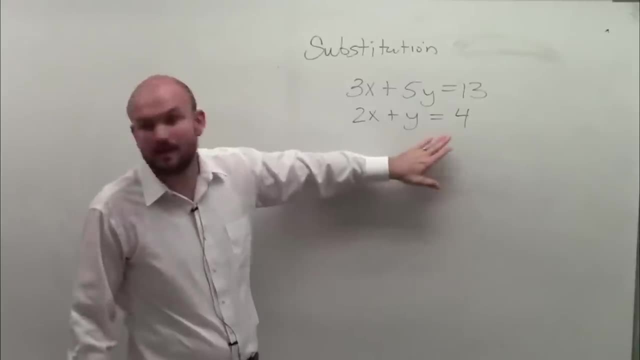 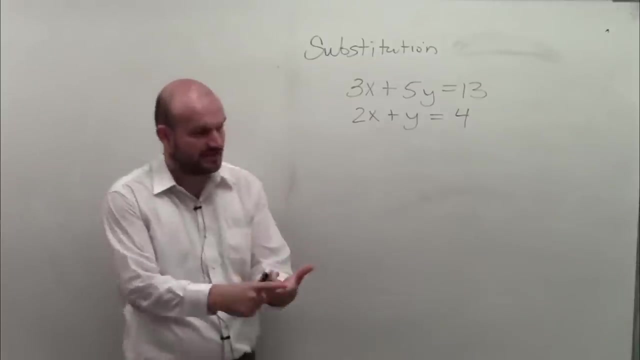 It's the same thing, But rather than getting out graph paper and trying to do all the graphing method, we can also use an algebraic method. OK, Now, the important thing is still: we're going to have our consistent, inconsistent solutions. 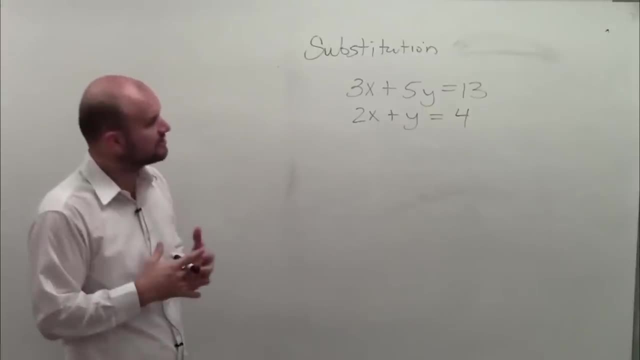 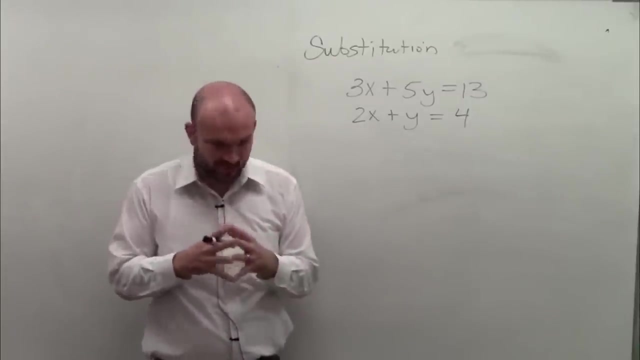 dependent and independent, And I'll kind of talk about those and what they mean algebraically. But in the substitution method we want to use a substitution method. The best time to use substitution is when You guys might want to write this down. 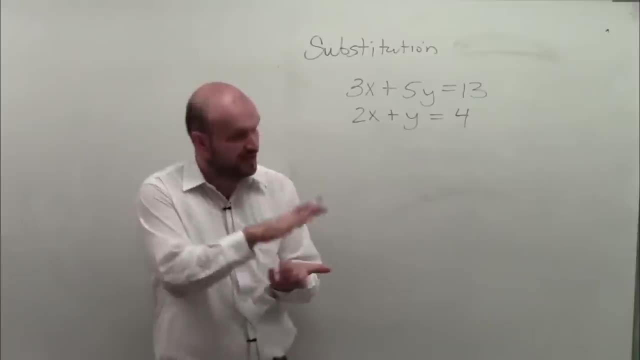 I'm not going to write it down for time purposes, But whenever you have a variable that is solved, or meaning any time you have a coefficient for one of your variables That is either 1 or negative 1.. So you guys can see right there. 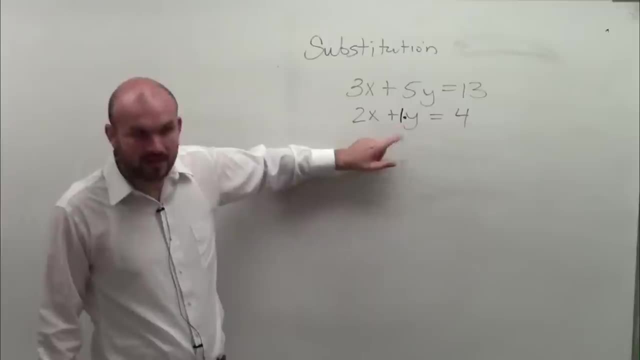 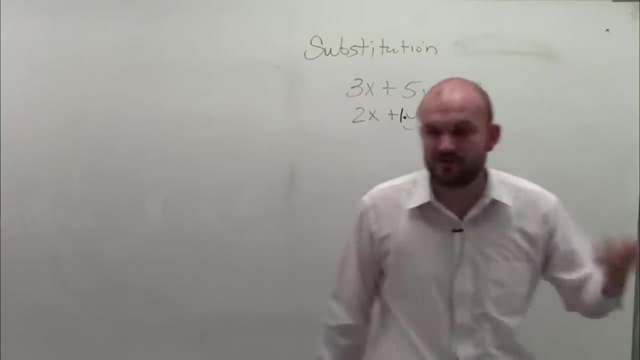 y has a coefficient of 1.. Right, So mentally in my brain, I'm going to want to use substitution. So any time you have a variable that has a coefficient of 1 or negative 1, Lizzy, it is going to be beneficial for you. 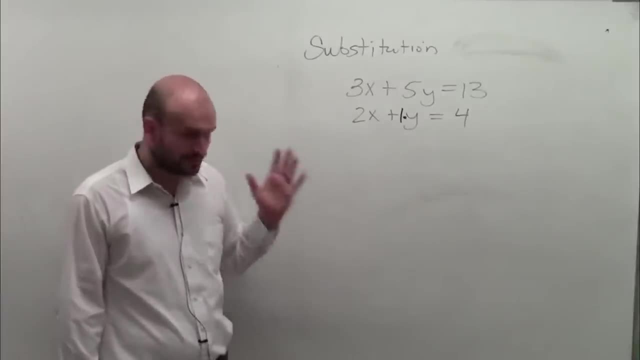 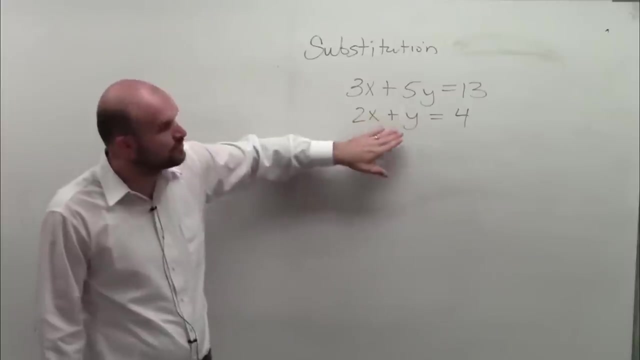 to use substitution Make sense. So how do we use substitution and why is it important when we have a coefficient of 1?? The reason being is because whatever variable has a coefficient of 1 or negative 1, and even if you have two of them. 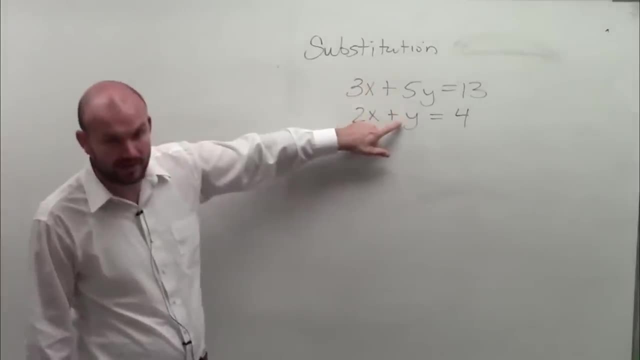 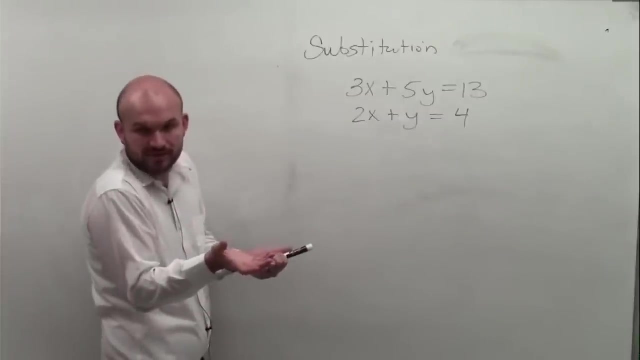 just pick which one you want to solve for. So let's say I have a variable that has a coefficient of 1, correct? So what I'm going to do is I'm going to solve for that variable, Because when it has a coefficient of 1,. 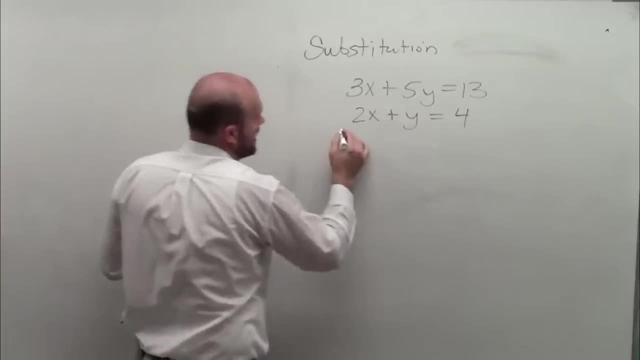 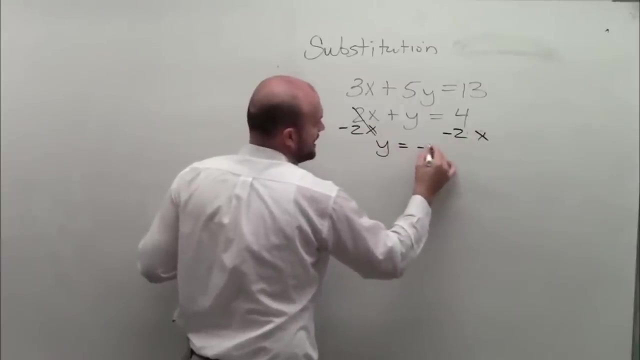 I don't need to undo multiplication or division, right? I just need to undo addition or subtraction. So I'm going to subtract a 2x from both sides. Therefore now I have y equals negative 2x plus 4.. So now, 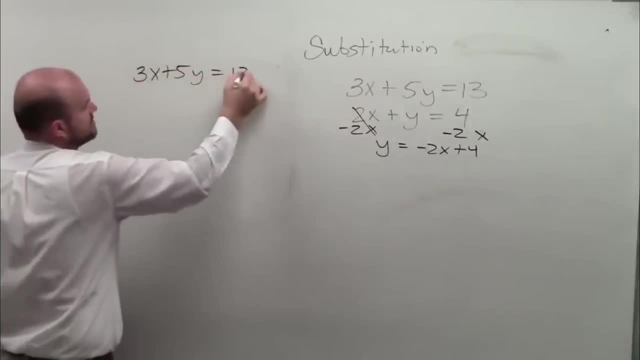 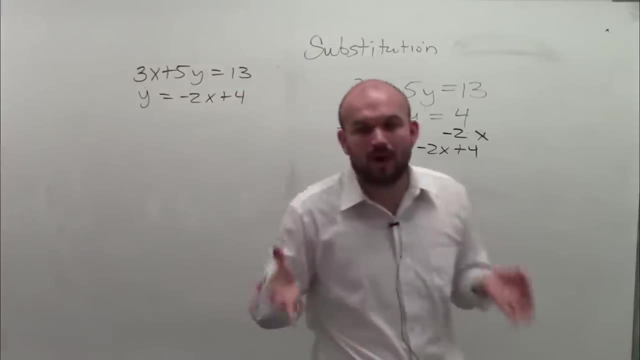 I'm just going to rewrite my system. It's 3x plus 5y equals 13, and then y equals negative 2x plus 4.. So basically, when we're doing substitution, we want to be able to have it written. 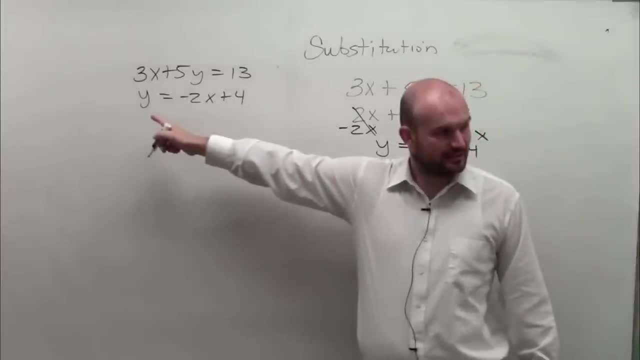 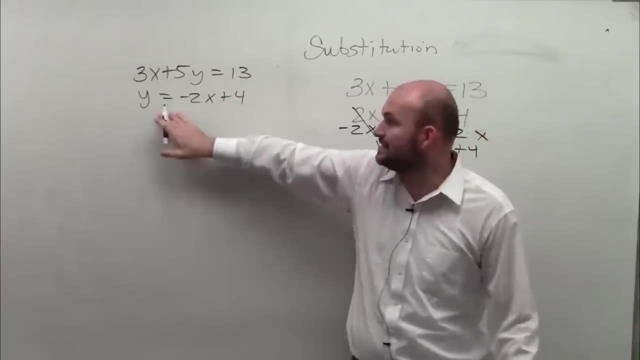 with a variable isolated, Alright, And you can do this when it's not equal to 1, but then you'd have to undo multiplication or division. So it's easiest when you have a variable that has a coefficient of 1.. So now 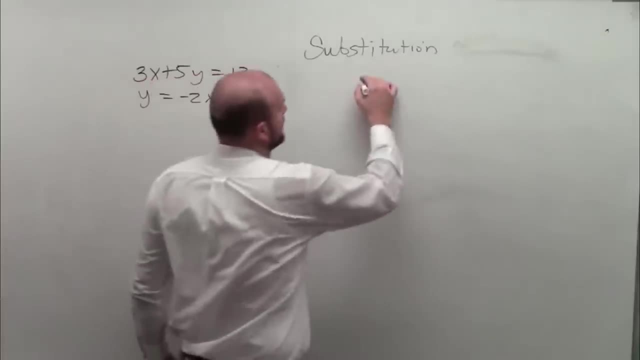 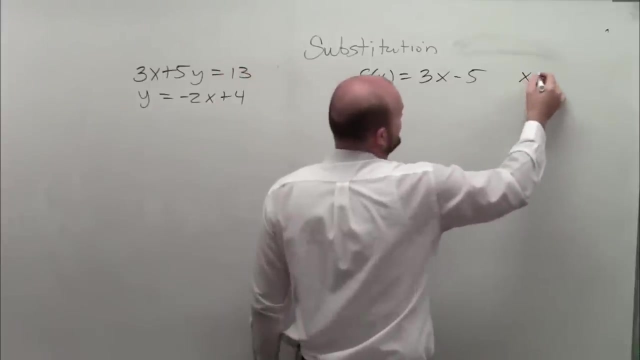 if you guys remember when we did functions, if I had f of x equals 3x minus 5, and I say, find when x equals 2, or I would say f of 2.. Now what else did we do with the 2?? 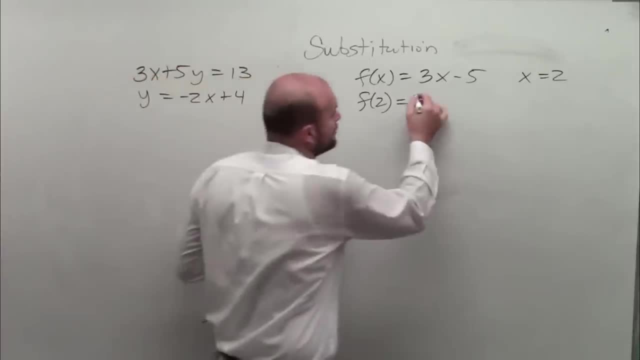 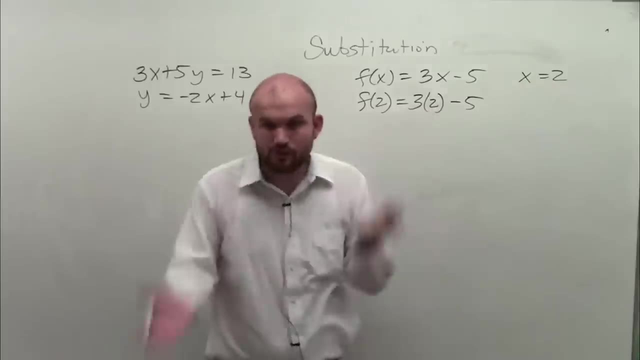 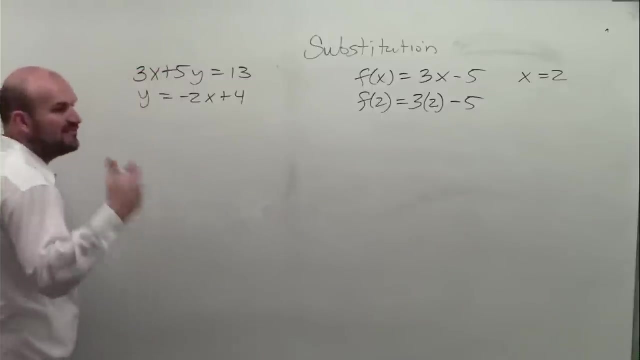 You put it in for the x right, So you did 3 times 2 minus 5, because x was equal to 2.. 2 was equal to x. You could replace them or substitute one for the other, correct? Now we're doing something. 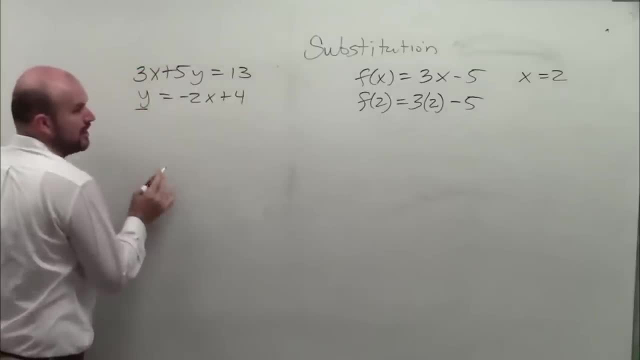 very, very similar. y is not equal to a number, but it's equal to an expression. But we can still substitute in that expression in for the variable. So that's exactly what I'm going to do: I'm going to substitute in my expression in for y. 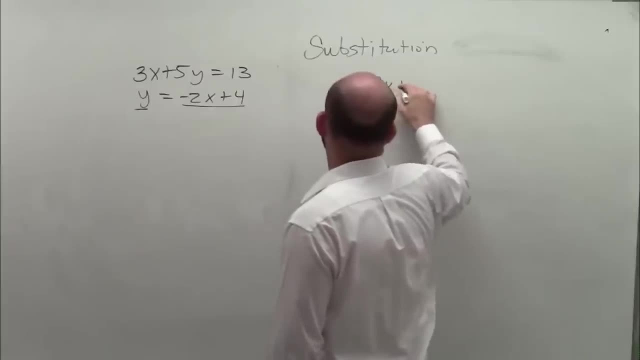 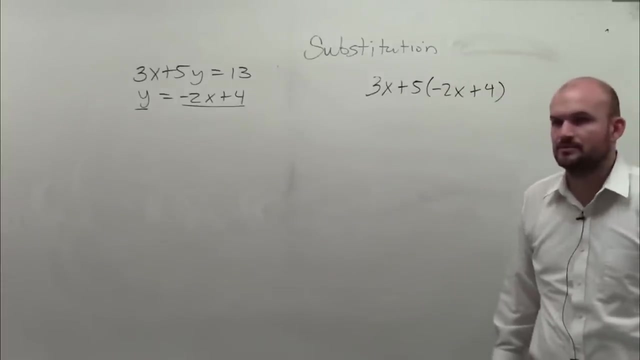 into the other equation. So I have 3x plus 5 times negative, 2x plus 4.. Okay, Jade, Got it. You doing, alright, You okay, Okay, Does everybody see? Does everybody see what I did? This is the big step. 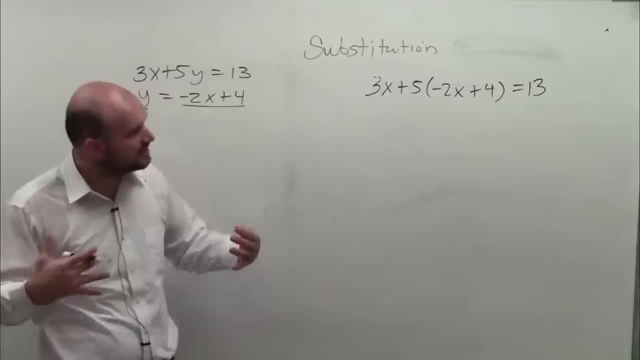 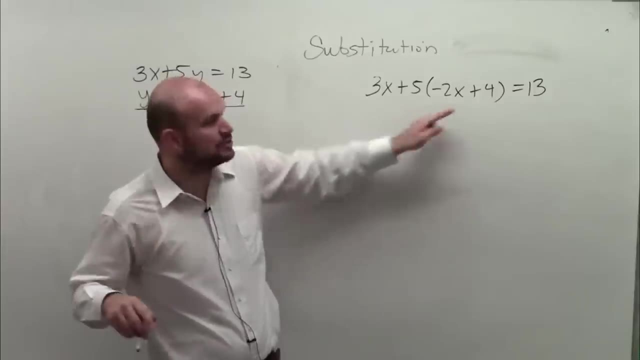 right there Now. the reason why that's so important is because now I have created an equation that only has one variable: x. Yes, it has two of them, but I'm only dealing with x. I'm not dealing with x and y's. 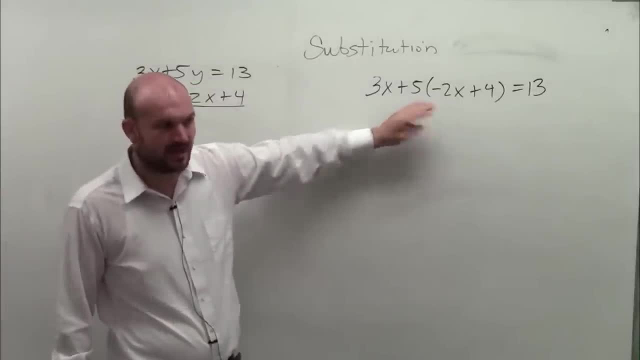 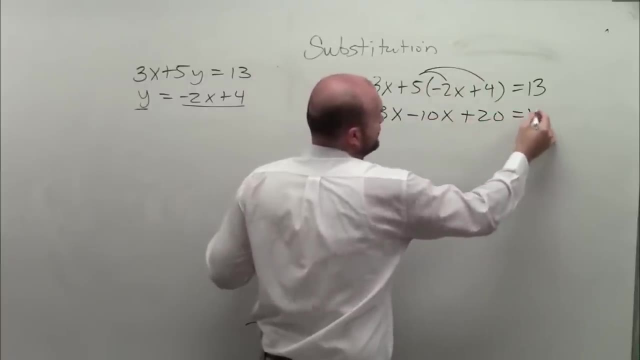 So now I can solve this. This is a multi-step equation. I can solve this, So I apply a distributed property. So I have 3x minus 10x plus 20.. 20 equals 13.. 3x minus 10x is negative. 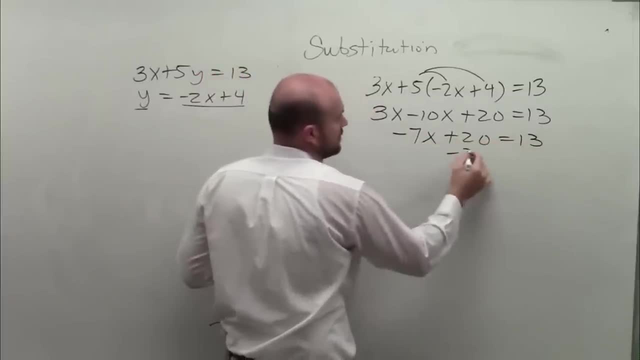 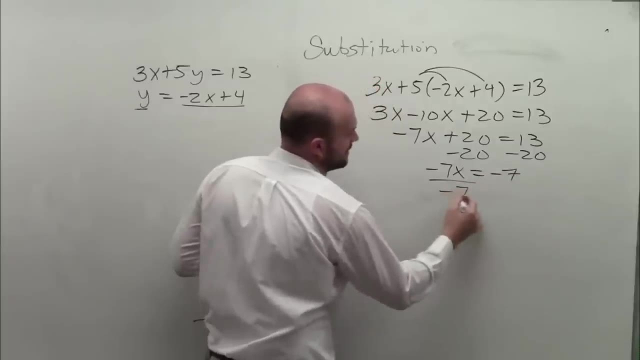 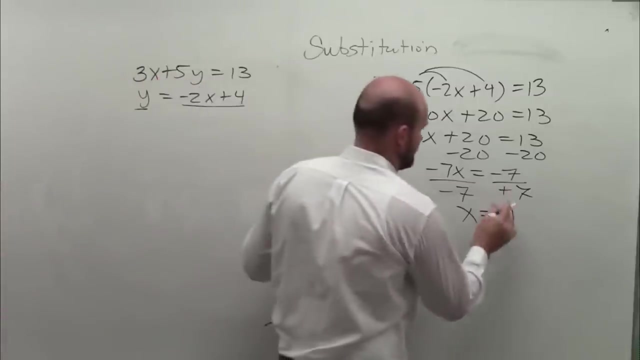 7x plus 20 equals 13.. Subtract: 20. Subtract: 20. Negative: 7x equals negative: 7.. Divide by negative: 7. Divide by negative: 7. x equals negative: 1. Positive: 1.. Thank you. 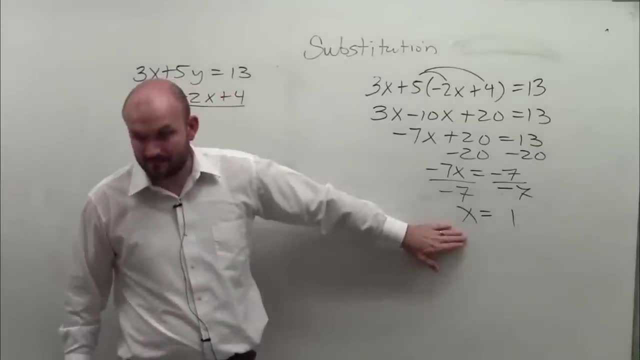 Negative 7 divided by negative 7 is positive 1.. So does everybody see that? Now I know the value of x. But again, when we're solving, remember when we did the intersection, We had an x and y coordinate where they intersected right. 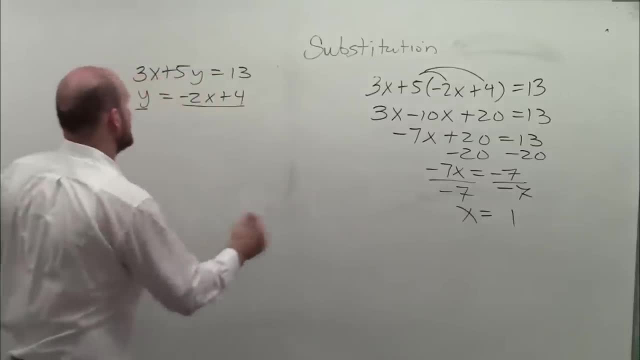 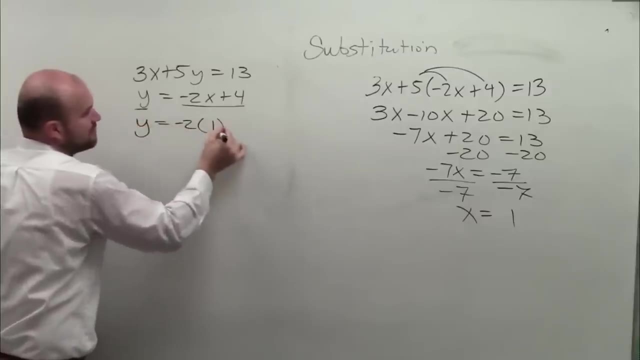 So we had x was equal to y, So now I'm going to take my value of x and plug it in for x. So I have: y equals negative 2 times 1 plus 4.. So y equals negative 2 plus 4.. 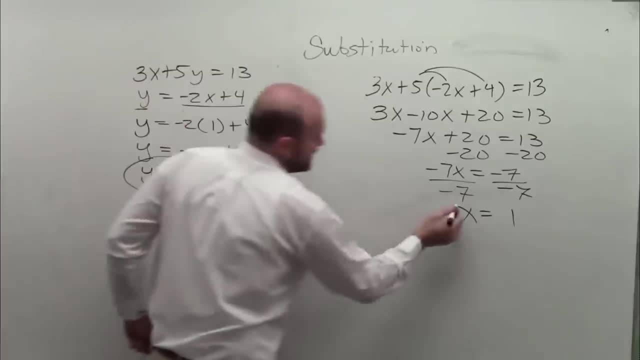 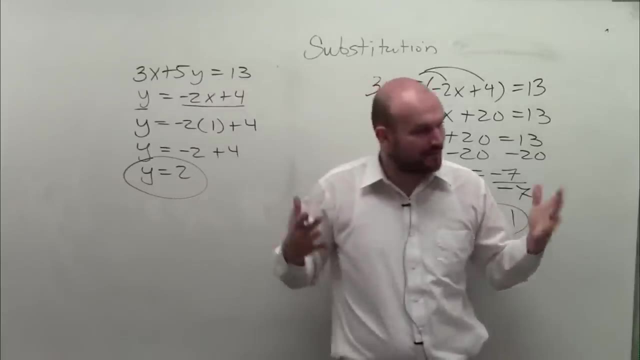 y is equal to 2.. So now I know the value of y and I know the value of x. Now on an equation. if you were to think about this graphically, if we know the x and the y coordinate, that represents where they intersect, right. 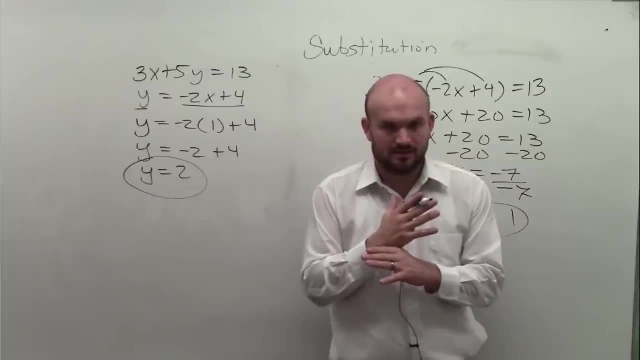 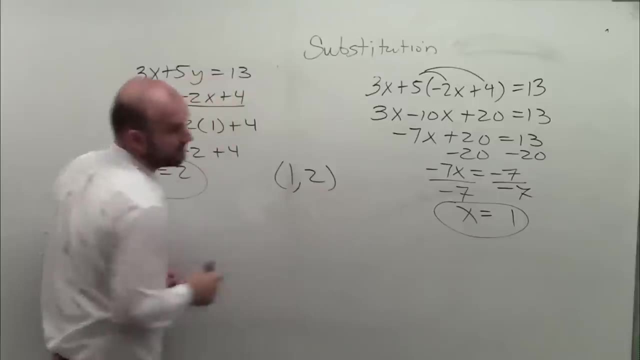 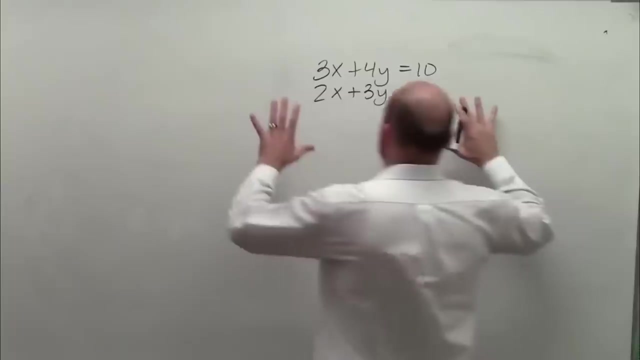 So then, what kind of solution Is this? consistent or inconsistent? Consistent, And they're going to intersect at the coordinate point. So it's a consistent, independent system, Because they only intersect at one point. You guys can see that I do not have any. 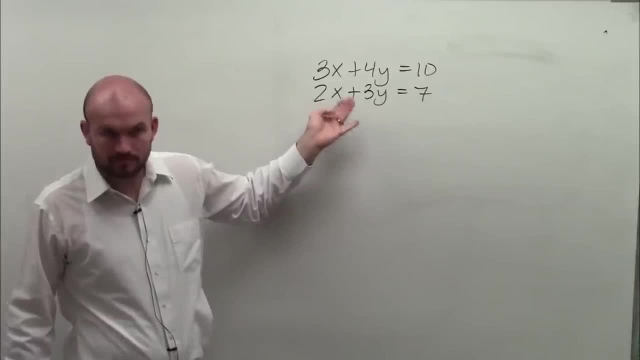 variable that has a coefficient of 1.. Correct, None of them have a coefficient of 1.. So if you're going to do substitution, you can still do substitution, but it wouldn't really be fun because then you'd have to solve for a y or an x. 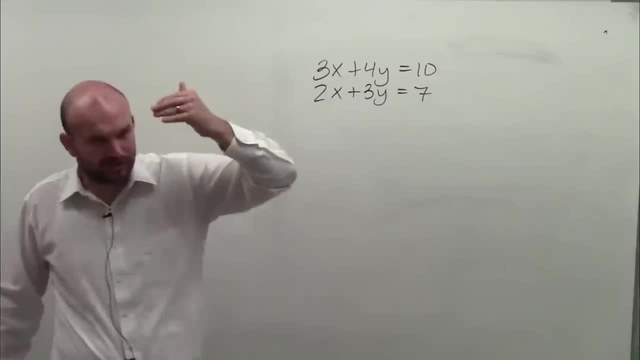 And if you guys kind of visually do that in your head, I'll go over this again with you. If you guys kind of visually do that in your head, you can see you're going to have some fractions And that's probably not going to be much fun to be working on. 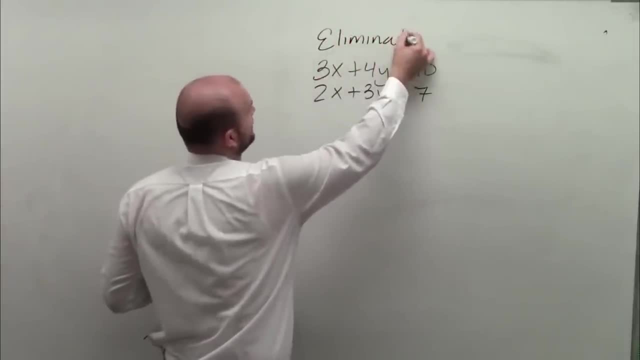 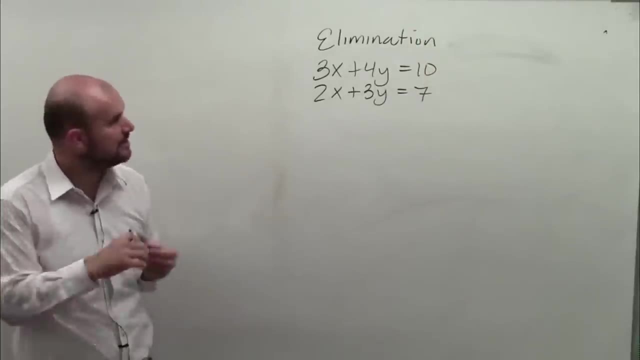 So the other method, which we call, is elimination, And using elimination, what we're going to do is add or subtract. add or subtract our equations to eliminate one of the variables. If I add or subtract these equations, if I add these equations, 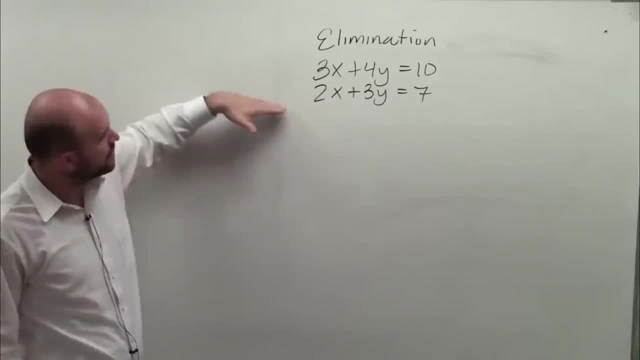 when we say eliminate, we want to get 0 as a coefficient, Right? So if I add these, do I get 0 as a coefficient. If I subtract these two equations, do I get 0 as a coefficient for any variable. 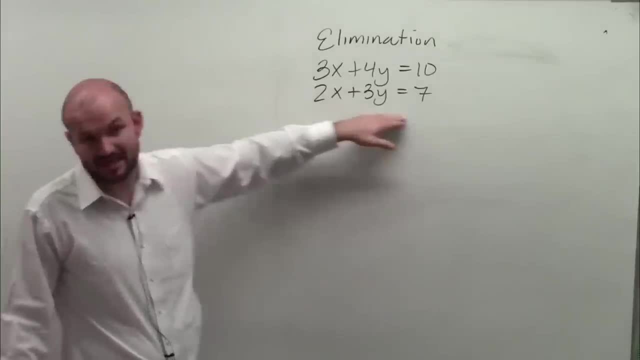 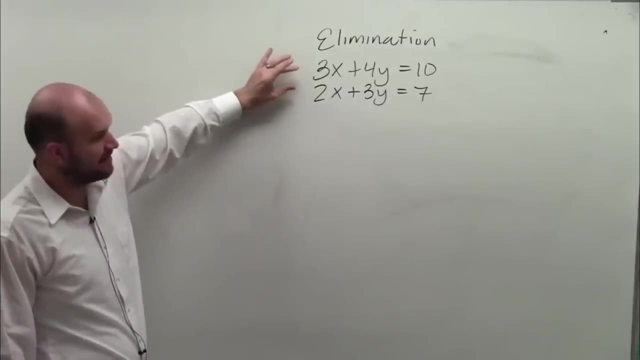 No, Sometimes that's going to work, but in this case that does not work. So therefore, I need to go to the next step, which is the hardest one. I need to find the common denominator or, I'm sorry, the common multiple. 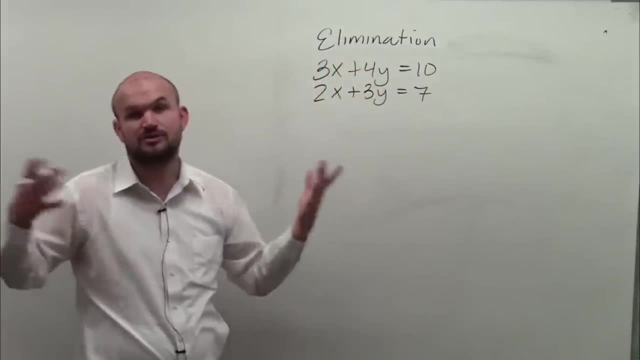 of 3 and 2 or 4 and 3.. Again, you can solve for x first or you can solve for y first. So what would you like to solve, for x or for y? Alright, so to solve for y. 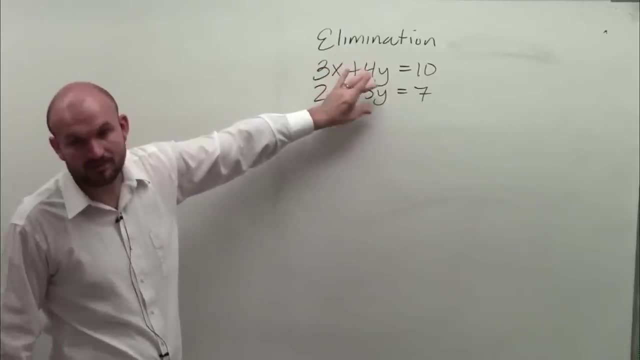 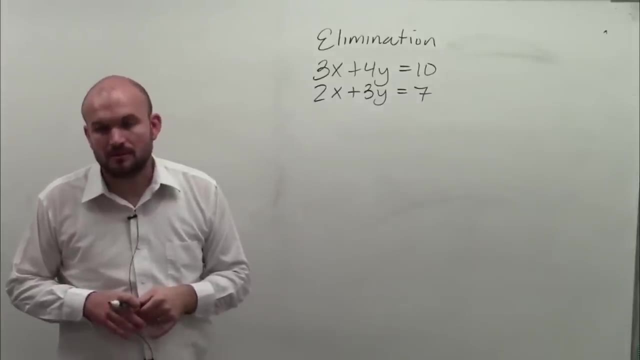 we have 4 and 3.. What is the common multiple of 4 and 3?? What is the smallest number that they both divide into 12.. Alright, would you like to add or would you like to subtract the equations? Okay, 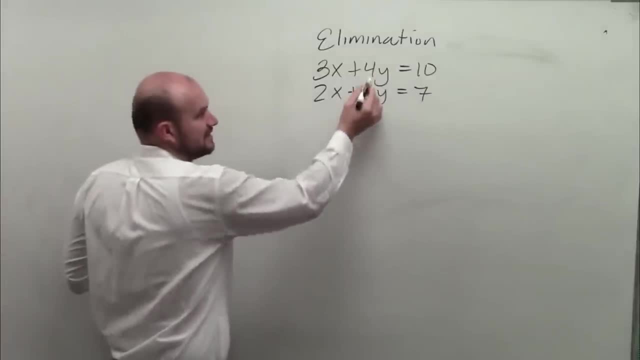 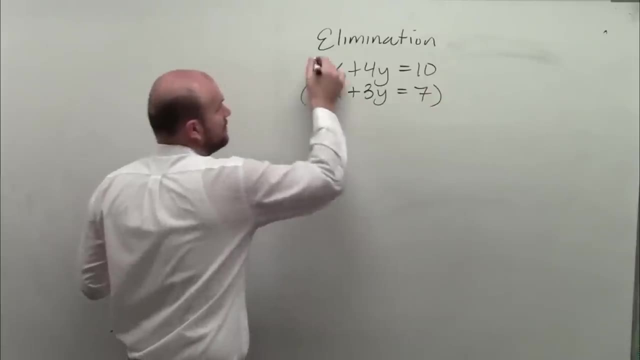 So there's different ways to do this. So he says: to get these, they add 12.. These both divide into 12, correct? So what I need to do is multiply them both so they'll be 12.. 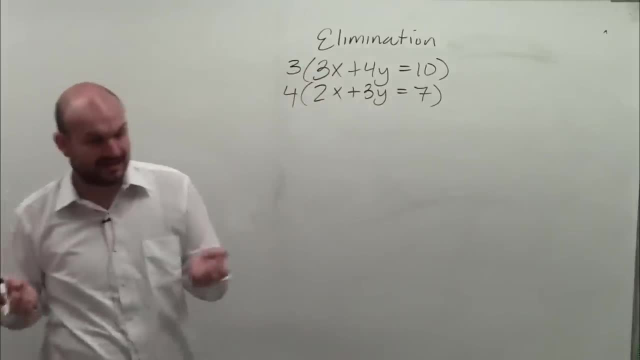 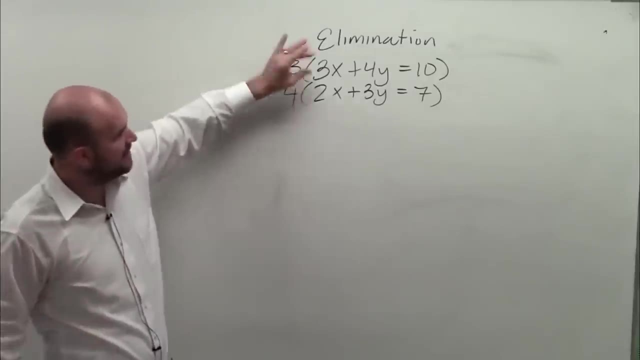 So here I'd have to multiply that by 4.. Here I'd have to multiply that by 3.. Now Cade did say he wanted to add, which I prefer adding. I don't like subtracting. Subtracting, I think, makes mistakes. 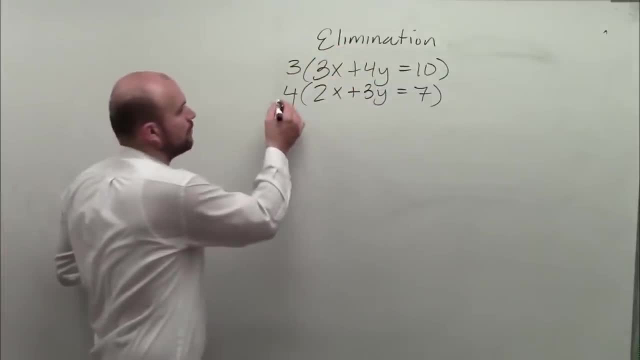 So if I'm going to add them, if I have 12y plus 12y, that's going to give me 24y right. So therefore I need to make one of them negative, Don't matter which one. 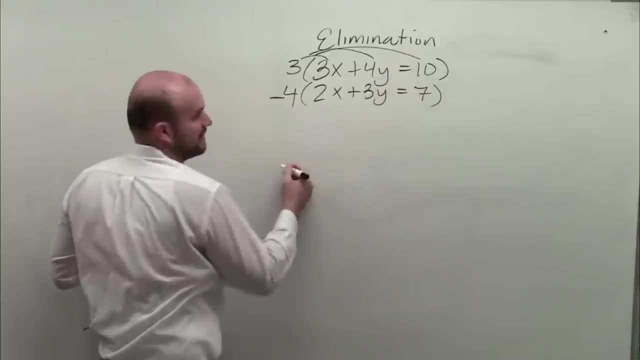 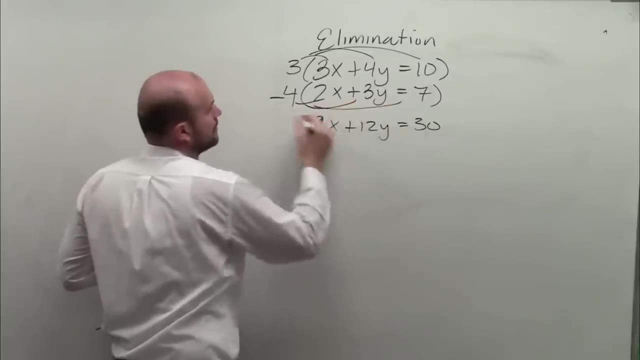 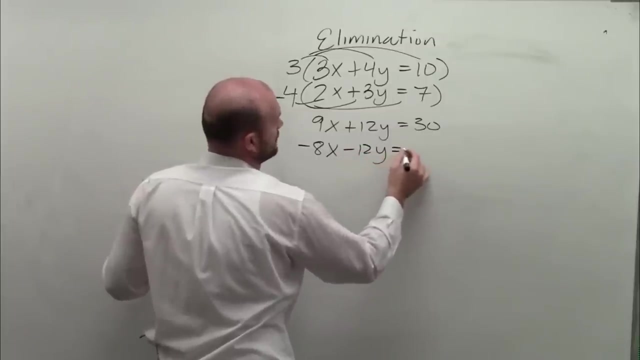 You just need to make: when you're multiplying, you've got to multiply everything. So this is 9x plus 12y equals 30. This becomes negative 8x minus 12y, negative 28.. Now I add them. 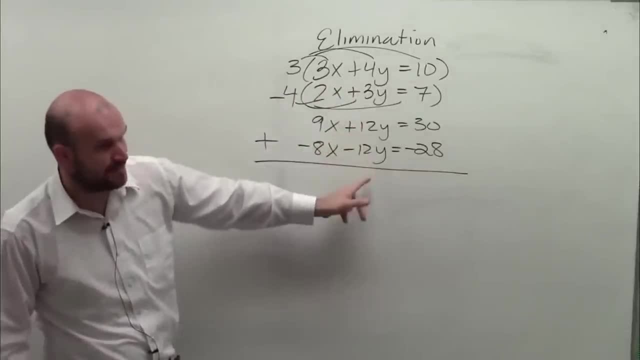 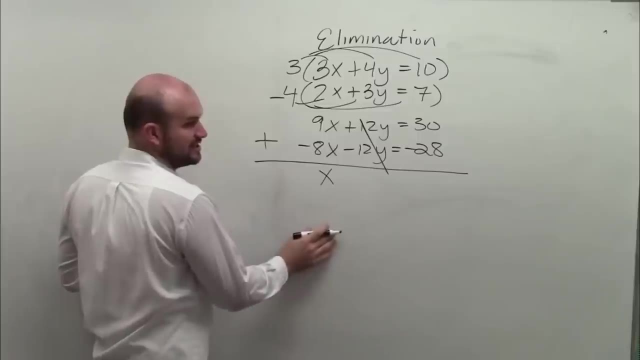 Alright, and I can add them because you can see, these are exactly the same. So therefore, 9 plus 8x is just going to be x. That goes to 0y, which is just 0, is equal to 2.. 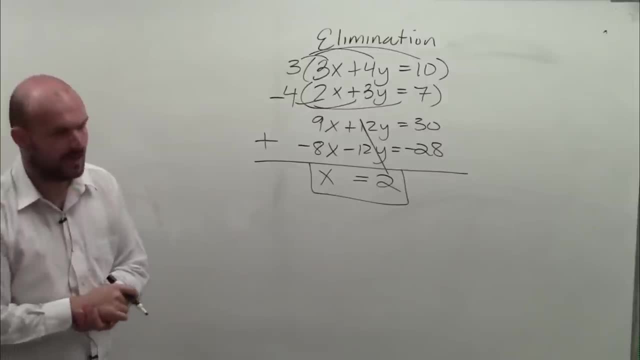 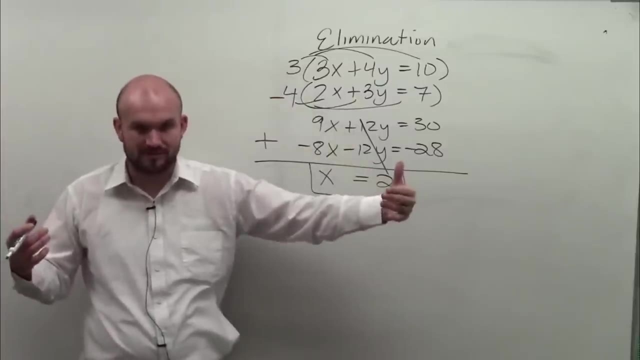 So now I've got my answer, Now we know what x is. Now we need to figure out what y is. But the problem, remember in substitution, how nice it was to have y solved right to plug the other one in. 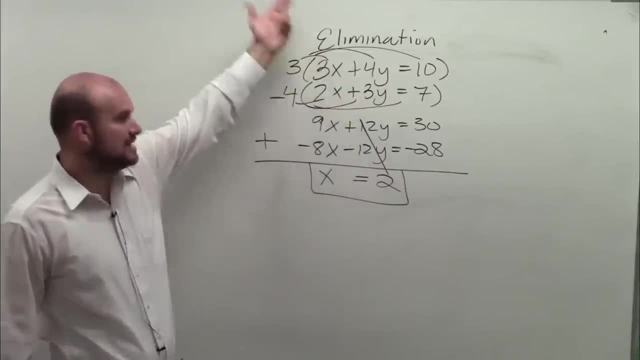 Here. we don't have one solved, So we just have to pick an equation. So, Jeremy, which equation You could use? that one or you could use that one, but obviously these are smaller numbers. So I'm going to say 3x plus 4y equals 10..